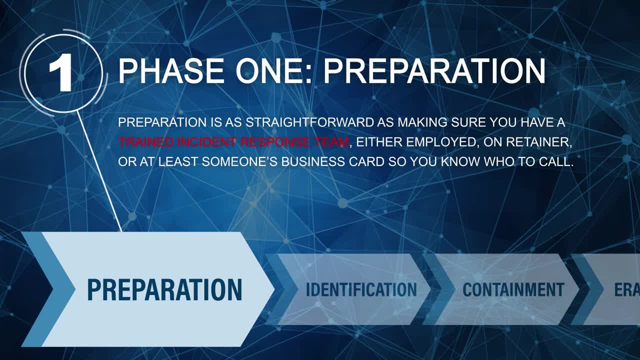 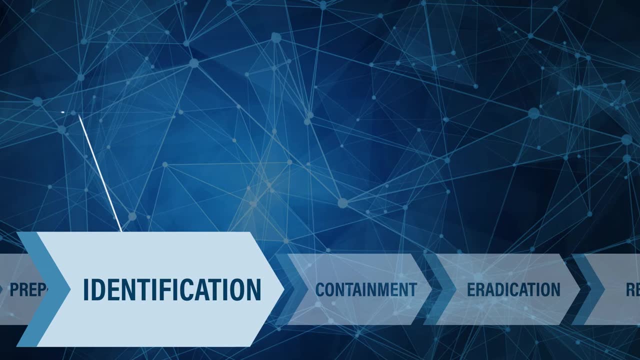 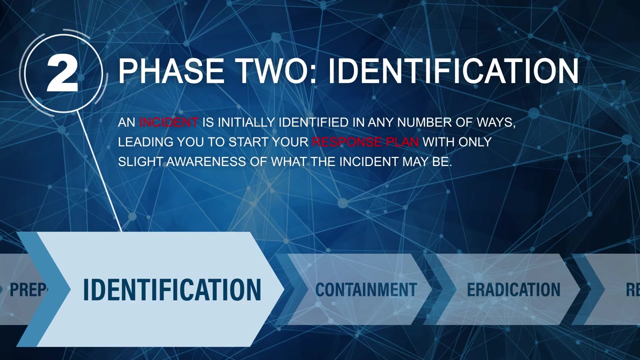 Preparation. Preparation is as straightforward as making sure you have a trained incident response team either employed on retainer or at least someone's business card, so you know who to call. Identification: An incident is initially identified in any number of ways, leading you to start your response plan with only slight awareness of 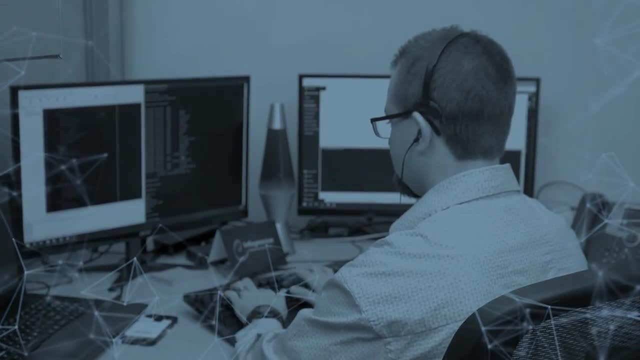 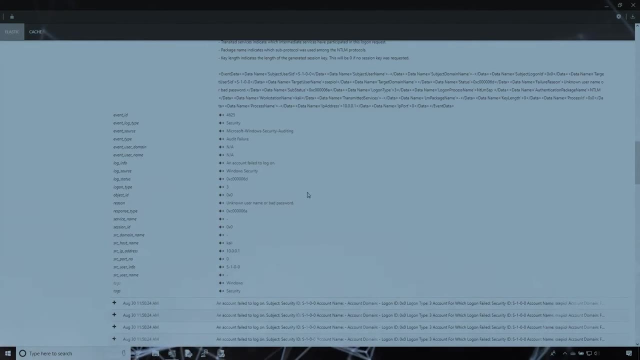 what the incident may be. The identification phase is meant to clear this part up. This phase also includes the investigation of the depth of the compromise, its source and its success or failure. Identification is done through review of log files- Lots and lots, and sometimes. 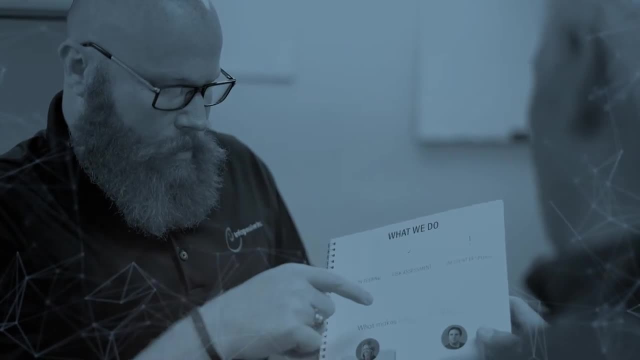 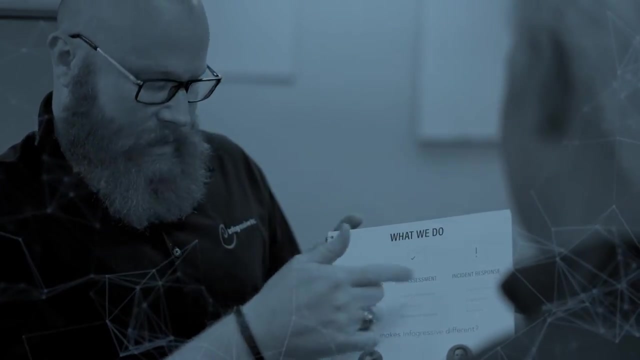 lots and lots and lots of log files. The important consideration at this point is not to disrupt any potential evidence of the incident. A well-trained and equipped response team will be able to rapidly parse log files, review forensic images and do so without damaging. 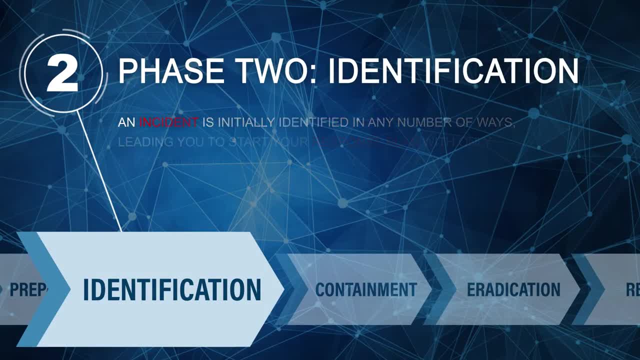 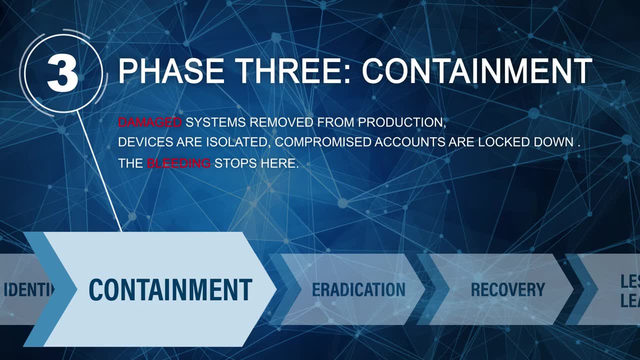 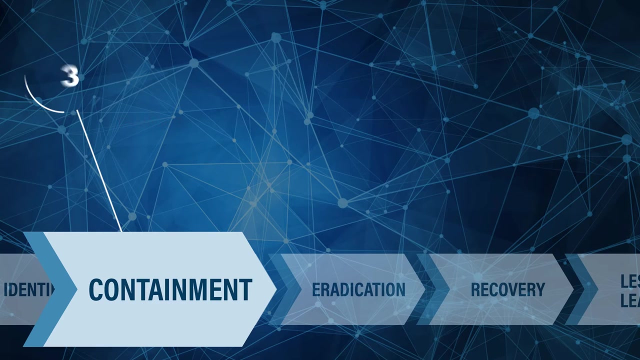 any evidence in the process, Containment. Containment often happens concurrently with identification or immediately following Damage. systems are removed from production, devices are isolated, compromise accounts are locked down. The bleeding stops here. Eradication. Eradication is exactly what it sounds. 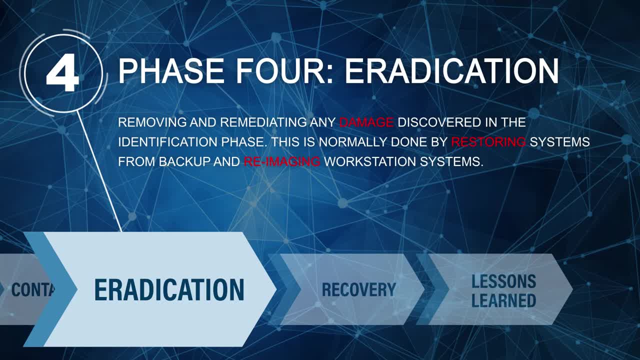 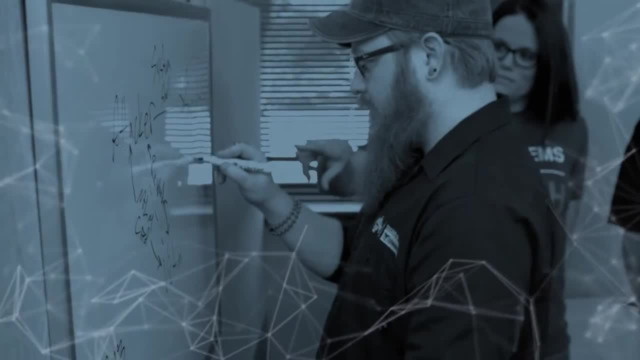 like Removing and remediating any damage destroyed in the identification phase. This is normally done by restoring systems from backup and re-imaging workstation systems. It's important to note that proper eradication of a cyber infection should be done by trained professionals. 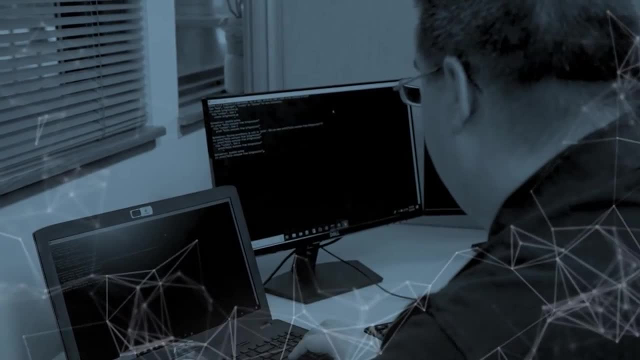 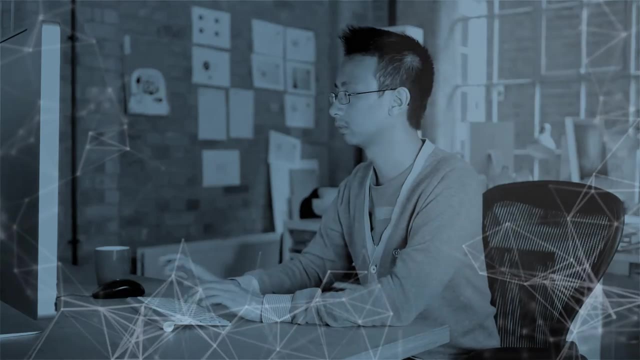 and should only be done after comprehensive investigation to the incident is completed. Time and time again, small organizations will be quick to delete, restore and re-image after the first sign of an incident, before they've learned how the attacker got in or how much damage was really done. In many 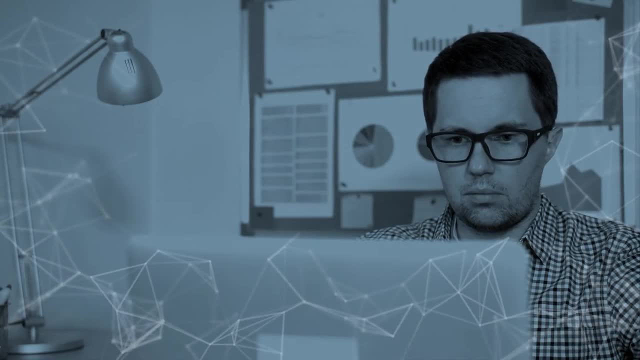 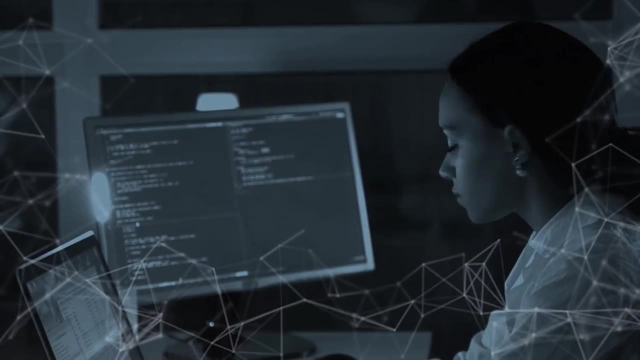 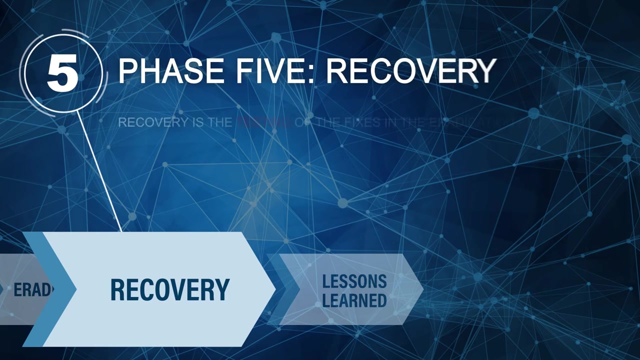 cases when systems are reset so quickly, the organization has no way of going back to learn what happened and, as a result, are often hit by the same type of attack again and again. Recovery- Recovery is the testing of the fixes in the eradication phase and the